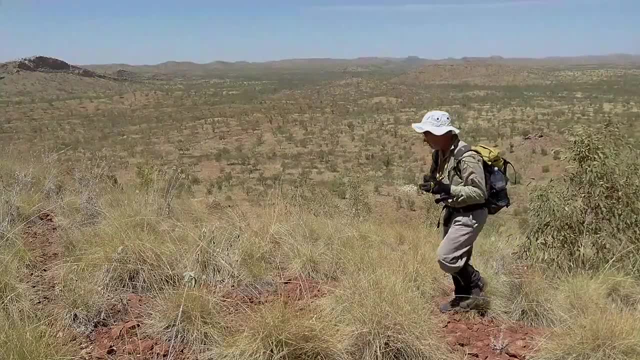 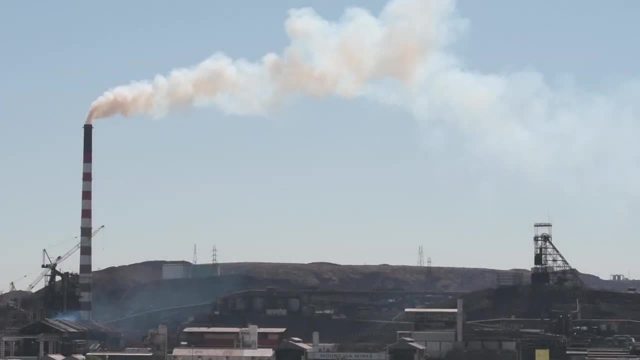 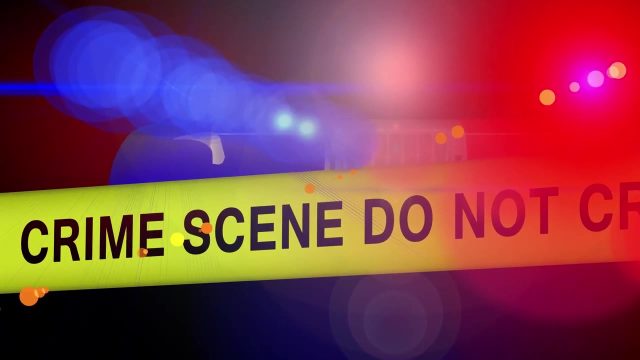 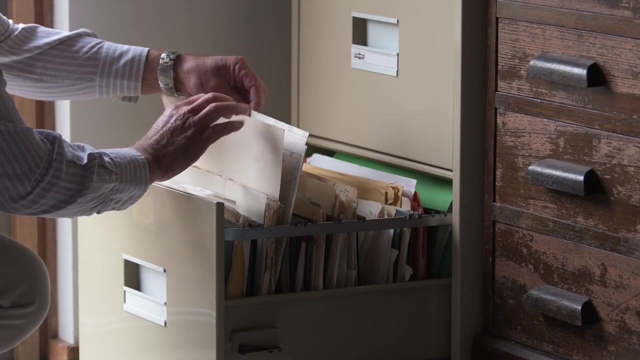 entirely indoors. I'm going to talk about mineral exploration geology, since that's what I do. The job of a mineral exploration geologist is to find new mineral deposits that will become the mines of tomorrow. I often liken exploration geology to cold case investigation. The thing you're looking for happened a long time ago. 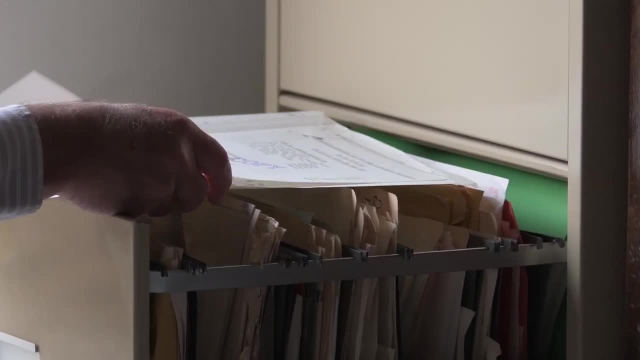 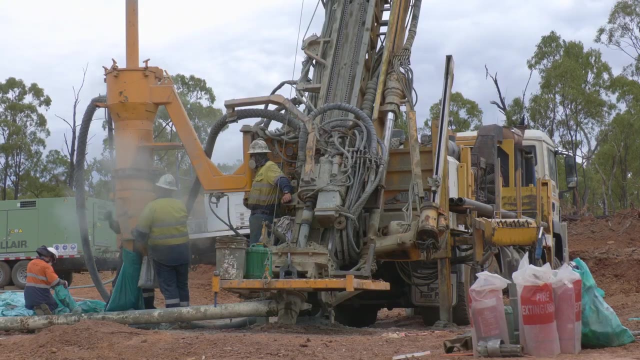 Most of the facts have been lost or destroyed or covered up. You develop a list of suspects, And some of them might look pretty good for a while, but then a single fact can give them a concrete alibi and knock them out of the race. 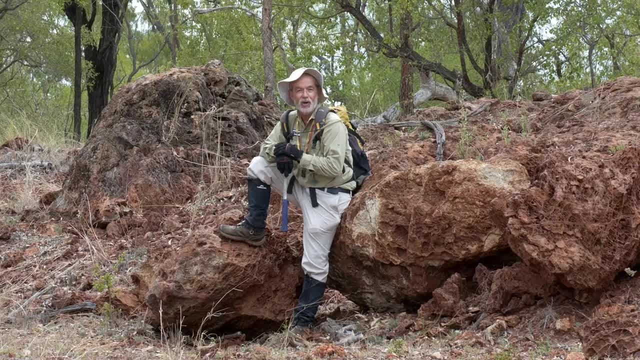 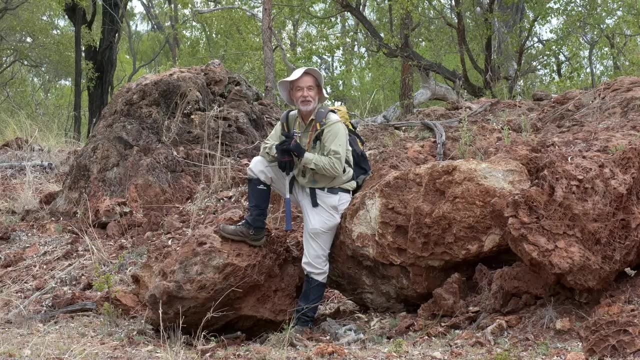 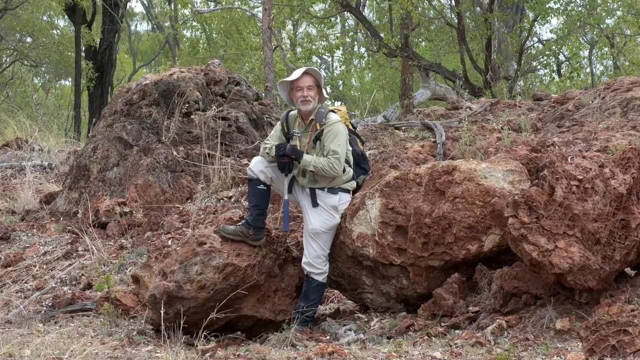 Sometimes it can take years and multiple groups of people working on the same thing before someone cracks the case. But if you're that person that cracks the case, the feeling of that discovery is just incomparable. That's why I do this job and that's why I go into the bush every day. 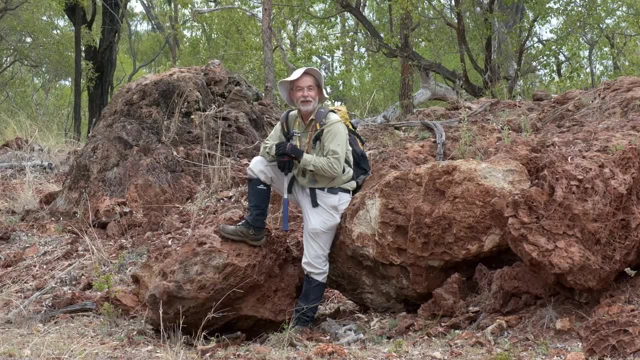 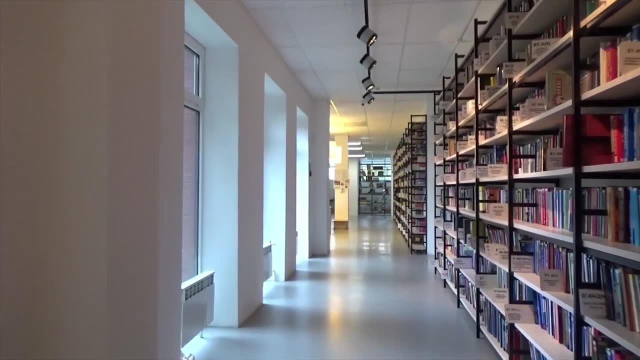 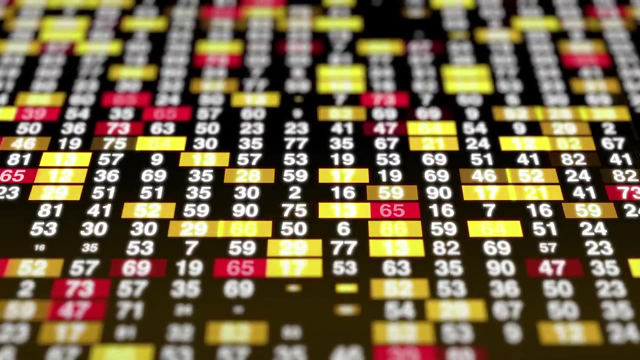 Because it never gets old. That thrill of discovery just never gets old. If you choose geology at university, you'll study basic science prerequisites- Physics, chemistry and maths- along with the geology subjects. You don't have to be a numbers nerd to graduate as a geologist. 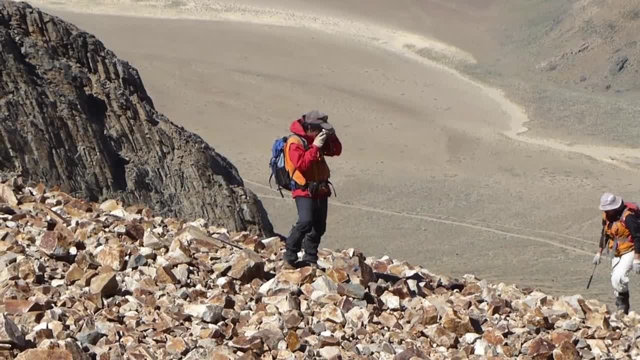 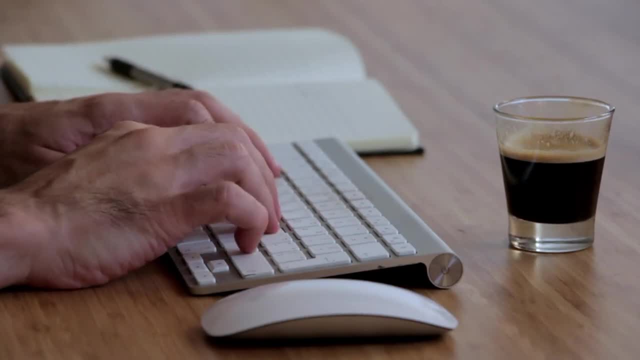 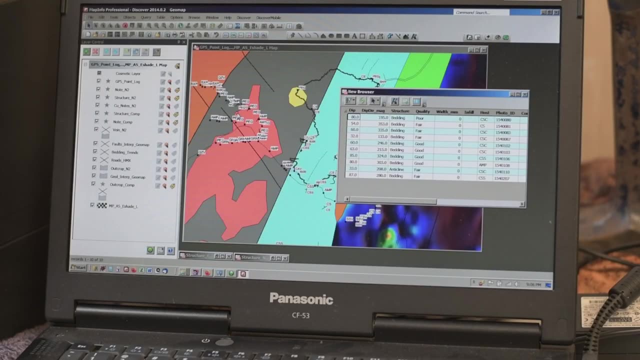 but having those basic science subjects under your belt will give you a much better understanding of the processes that make the rocks you study. Having an affinity for computers will also help you when you're compiling, interpreting and presenting the data you collect. Modern day exploration geologists have access to a staggering array of data from automated machines. 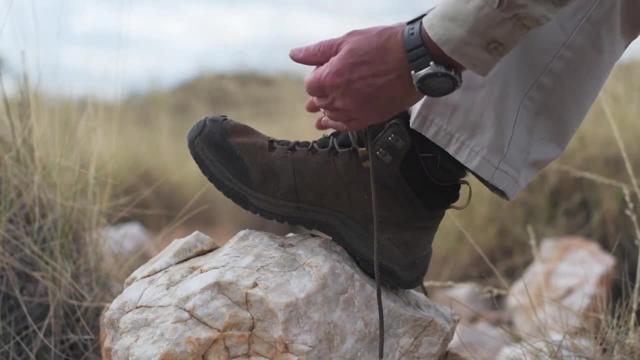 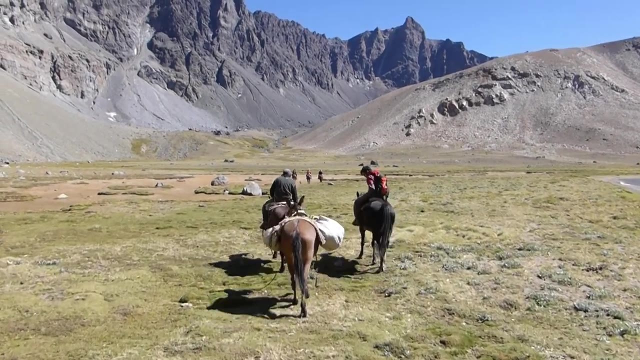 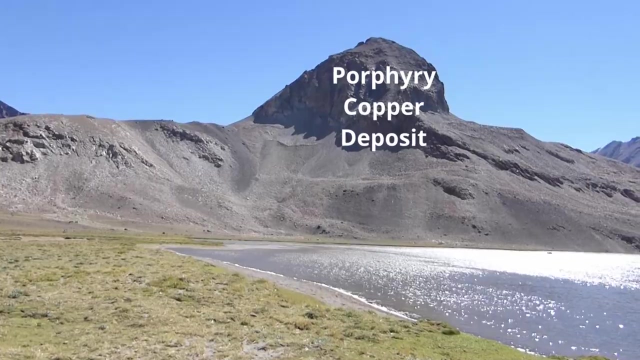 But field boots are still the most effective tool for interpreting that data, So you'll need to enjoy working outdoors. You get to go to some really wild and interesting places that other people will have to pay stupid amounts of money to go and do. You're getting paid to do it. That's pretty hard to beat in my book Now sometimes 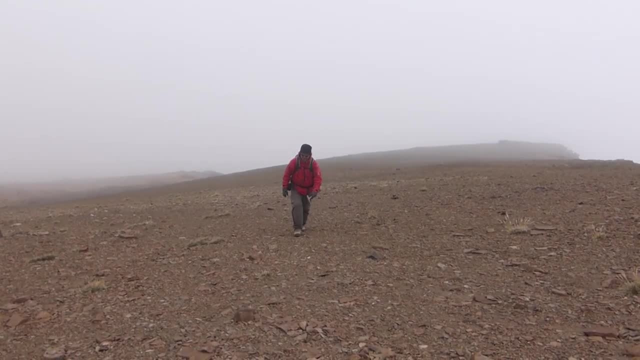 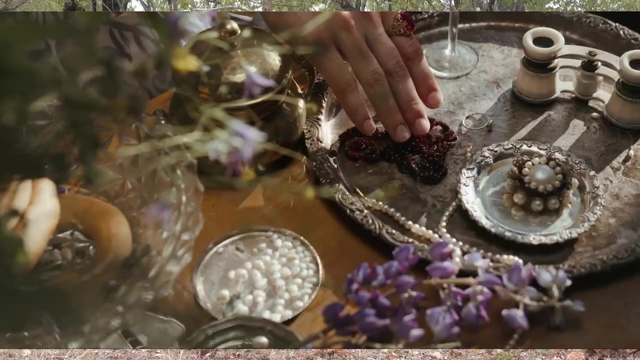 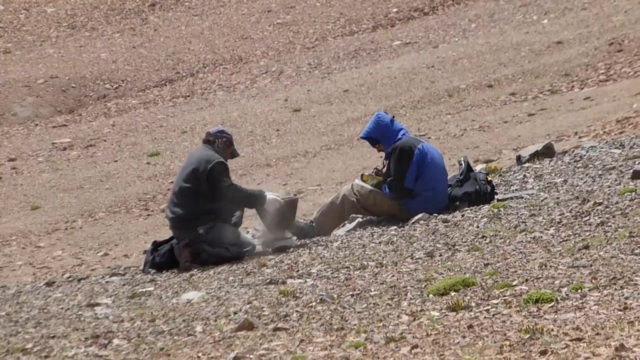 you're going to go to places that are not so nice, but that's a harsh reality of life. Humans want the things that geologists bring- the gold, the lead, the zinc, the silver, all those things- but nobody wants a mine in their backyard. So the bottom line is: exploration usually gets done.